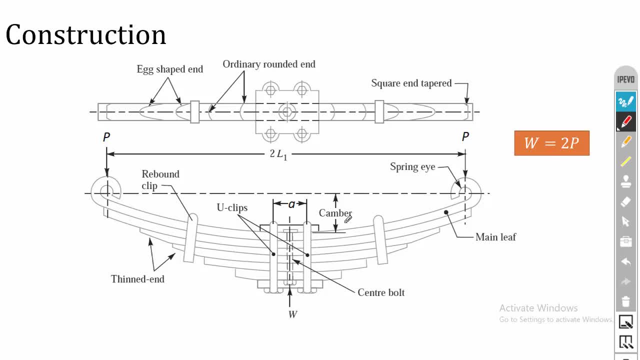 it is loaded, the leaf spring will absorb the high amount of loads. so the first leaf is called as main leaf or master leaf. after the main leaf, full length leaf size there, okay. so the second leaf is called as full length leaf or extra full length leaf. okay. 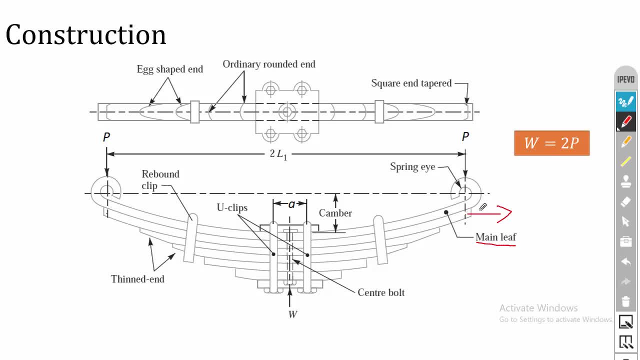 so you can see that the length of the leaf is full, so that is why it is called as full length leaf. after the full length leaf, we have graduated length leaves. okay, so this? all leaves are held together by these rebound clips. okay, so this rebound clips are used to align the various leaves. and in the center we have 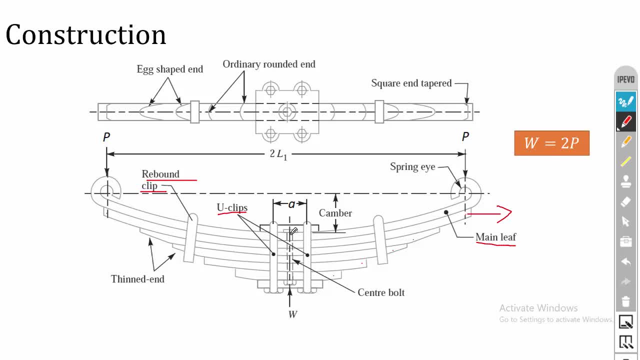 a U-Clip. so this U-Clip is actually used for two purposes. one is for keeping all the leaves in position, and also here your axle will be fixed in this direction. So the axle is fixed in the u-clip, so the load is applied throughout the u-clip. 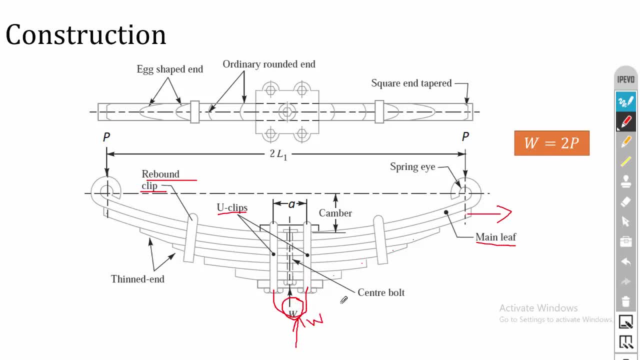 So here the applied load is considered as W and while designing the leaf spring we are going to assume that we are going to fix the leaf spring at the center and we are going to split the load into two. So imagine that we are fixing it in the center so that it will act like a cantilever beam. 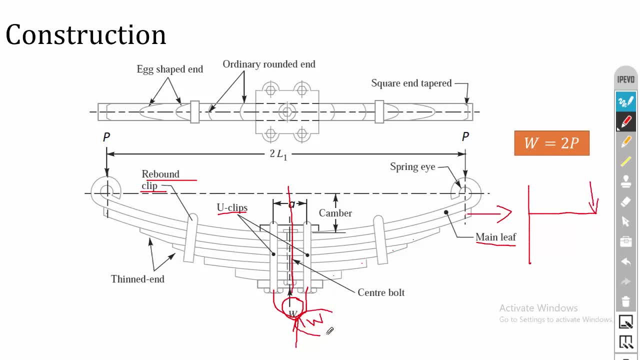 and the load is applied like this. So this W is splitted into two, that is P is equal to W by 2.. So that is W is equal to 2P, so P is equal to W by 2.. So while designing the leaf spring, we are going to focus on only one side of the spring. 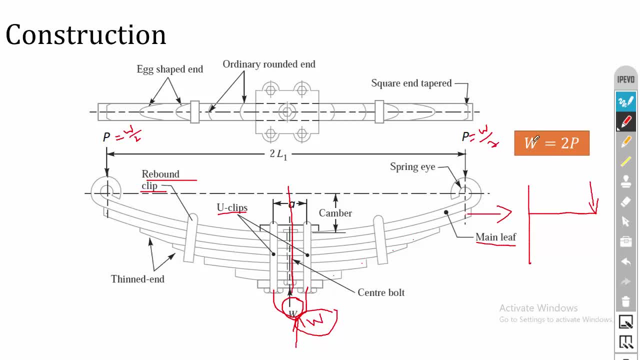 not the other side. Ok, So that is why I have splitted the load into two parts. So when you are combining the two loads, then we will get the overall design. So this is the construction of leaf spring. So here the 2L1 is the length of the spring and the camber is the initial deflection provided. 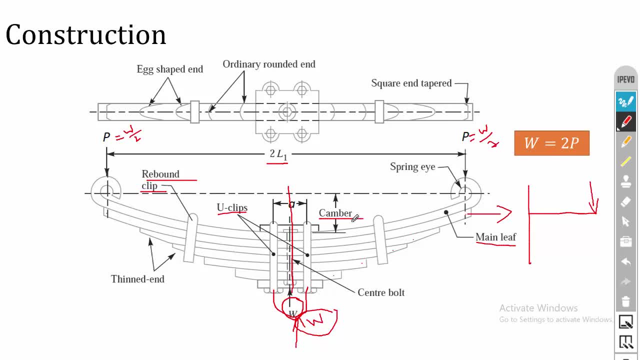 So the initial deflection provided in the main leaf is called as camber. So this deflection is to absorb high amount of load. so pre-stressing the process is called as pre-stressing. So pre-stressing means before applying the load, we will apply the stress in the opposite. 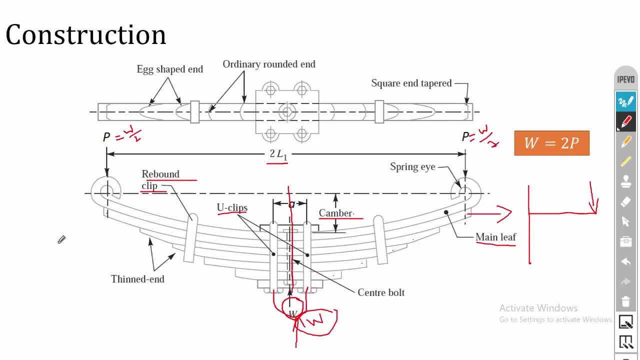 direction. So when it is loaded the load will act in the opposite direction and the opposite stresses will get neglected. So that is called as pre-stressing, And the distance between these two bolts- U bolt- I mean the distance between the U bolt- is called as A, that is bandwidth. 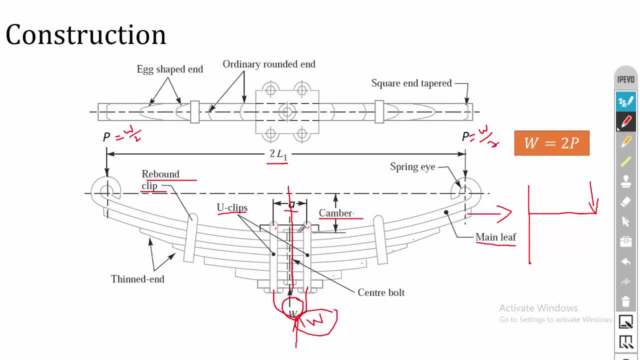 Ok, So to design this U bolt, the spring will act like a rigid structure. that is why it is called as bandwidth. and while designing the spring, we have to neglect this region, because this region will act like a solid material. it will not have elastic properties. 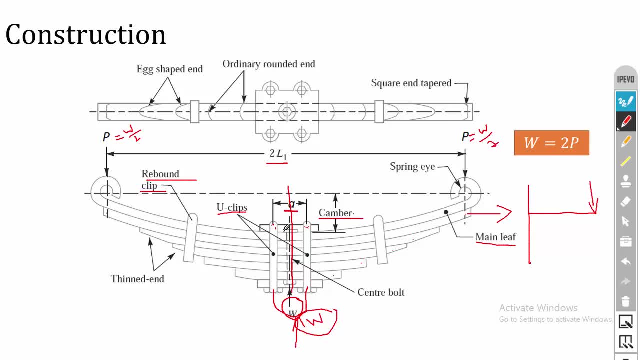 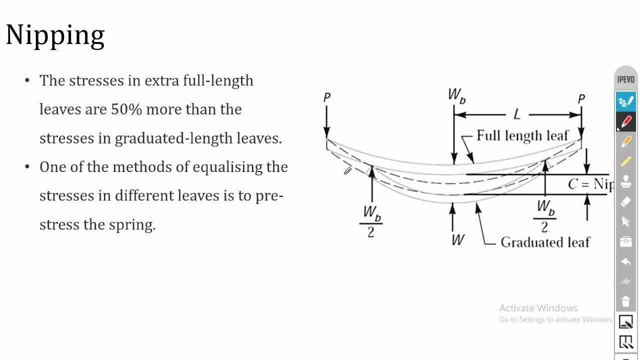 So that is why it will not absorb the load and it will not provide the stiffening effect. So that is why we have to neglect this bandwidth. The next one is nipping. So, as I told earlier, we are providing pre-stressing to release the additional stress applied. 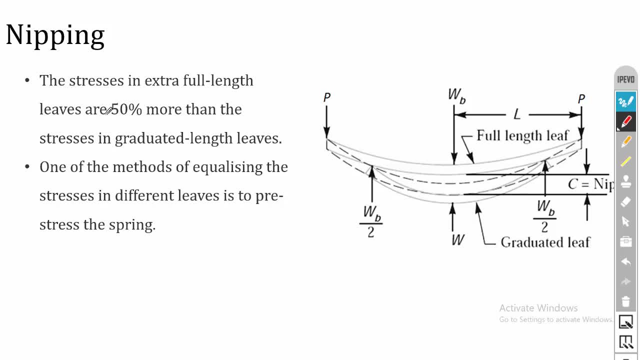 And in the leaf spring the full length leaf carries 50% more than the stresses applied in the graduated length leaf. So that is the first leaf is carrying 50% more stress than the remaining graduated length leaves. So we have to equalize the stress in different leaves. 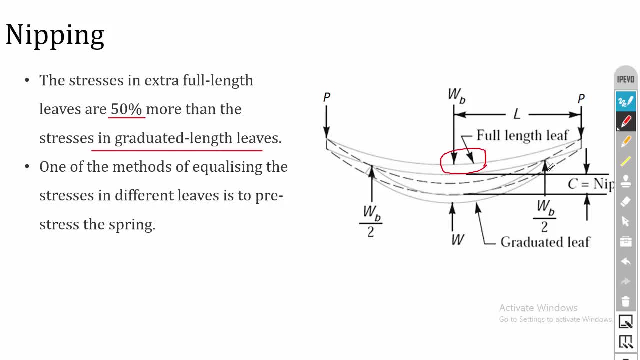 That is why pre-stressing process is used and here in this full length leaf, we are providing some gap between the full length and the graduated length leaf So to absorb the additional stress that is carried by the full length leaf. And this initial gap is called as nip C. that is equal to nip and the process of providing. 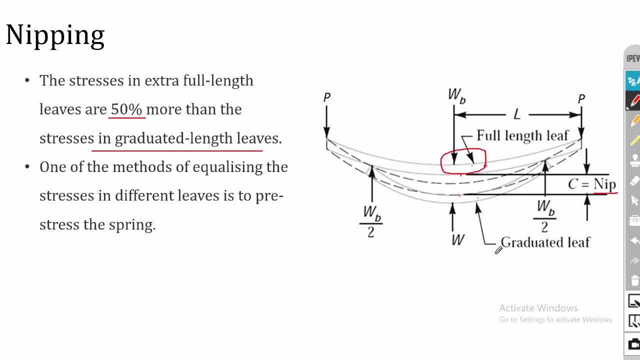 the gap between the full length leaf and the first graduated length leaf is called as nipping. So this process is very important for leaf spring. So nipping is very important for leaf spring to really normalize the stresses acting on the various leaves. So the design procedure, 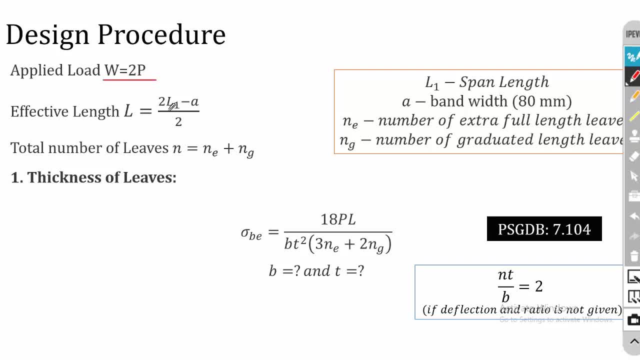 So initially in the problem they will specify the total load applied, that is W, And we are, when we are designing we have to focus only on the load, P, And we know that the load is equally divided into 2. that is why P is equal to W divided by 2.. 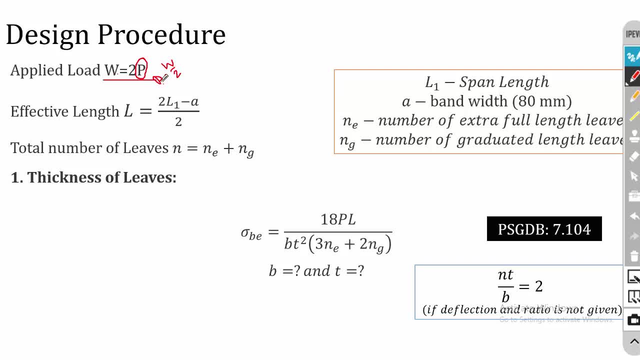 So we are going to use the P in all our design calculations. So at the initial stage you just calculate the P, that is, total load divided by 2. Then the effective length. So, as I told you earlier, we are going to neglect the distance of bandwidth while designing. 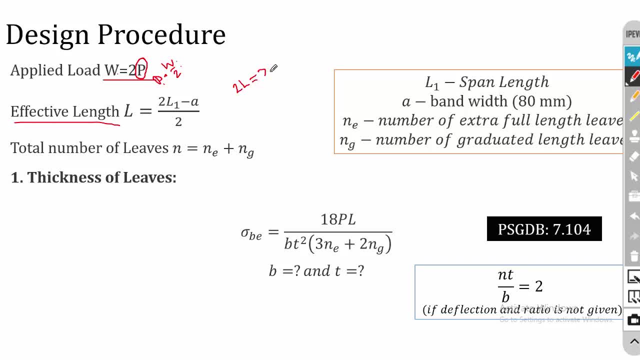 So the effective length is: 2L is equal to 2L1 is the overall length and minus A. So here the 2L1 is the overall length, 2L is the effective length, because we are going to minus the bandwidth here. 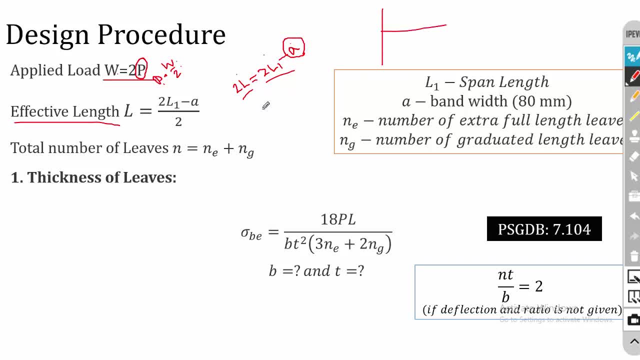 So the meaning for 2 is, as I told you earlier, we are going to split the spring into 2.. So that is why we have used 2 here, and when we are considering for one side, then we can put: L is equal to 2L1.. 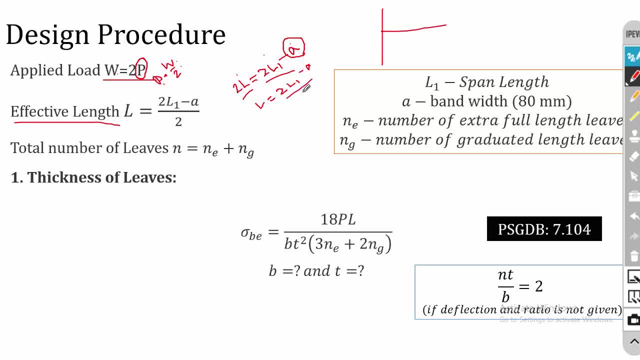 Okay, 2L1 minus A divided by 2.. So 2L is the effective length for both the sides and L is the effective length for one side of the leaf spring. So at the initial stage you have to calculate the load applied on one side and the effective. 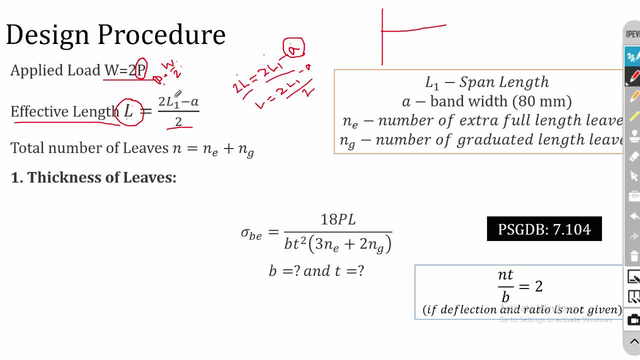 length on the one side. So don't confuse the L1 and L value. Mostly in the problem they will give the span length. that is, the 2L1 value will be given in the problem From the 2L1 value. by substituting the value of bandwidth we have to calculate the length. 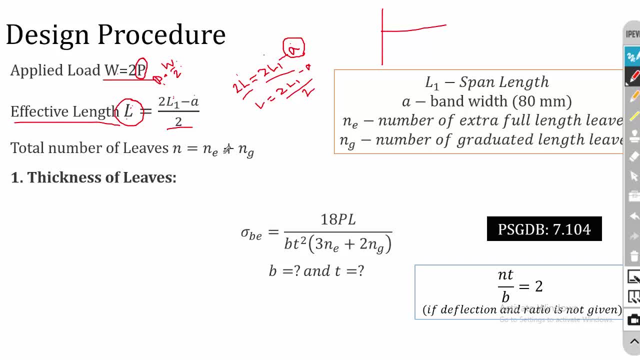 of the spring. And remember that in some of the cases the bandwidth may not be given. So if it is not given then we can assume a bandwidth value of 80 mm. Then the total number of leaves, So N, is equal to extra full length leaf or full length leaf plus the graduated length. 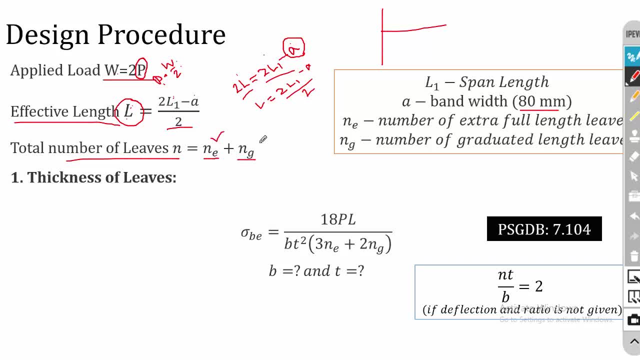 leaf. So total number of leaves is the summation of extra full length leaf and the graduated full length leaf. Then the problem. they will specify that how many number of leaves the spring has or otherwise. we can assume any at 7 or 10 or 15, based on our load requirement. we can assume the value. 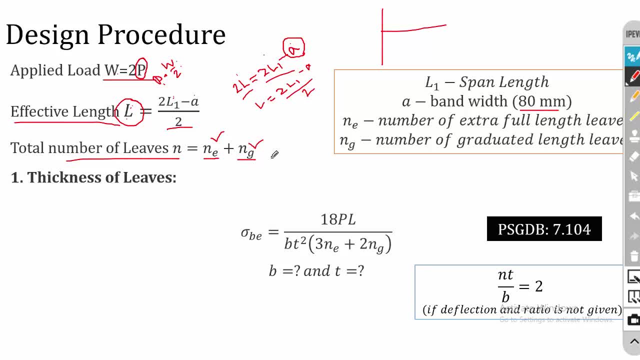 But in most of the cases the number of leaves will be given. So the first step of the design procedure is thickness of the leaves. So we have two equations for calculating the stress. one is sigma BE and the other one is sigma BE. So if you take the data book, page number 7.104, you will have two equations. 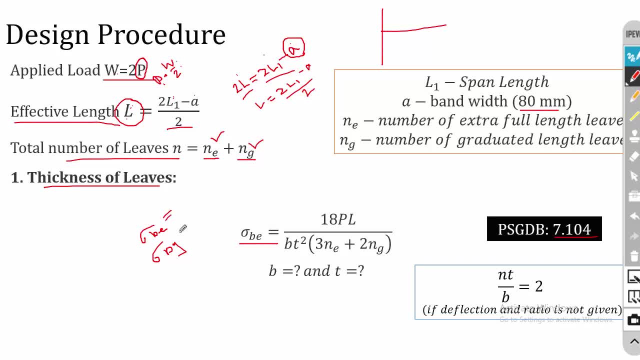 So sigma BE is stress acting on the extra full length leaf and sigma BG is the stress acting on the graduated full length leaf And, as I told earlier, we are going to consider the spring as a cantilever beam, So bending stress will be acting. 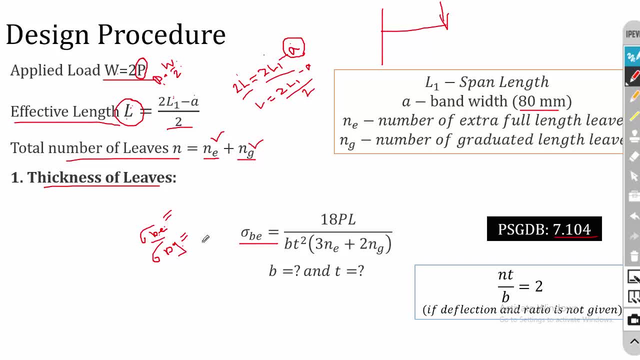 So that is why I have used B. E is for extra full length leaf and G is for graduated length leaf, And in the previous slide I told that. So that is why I have used B. E is for extra full length leaf and G is for graduated length leaf, And in the previous slide I told that. 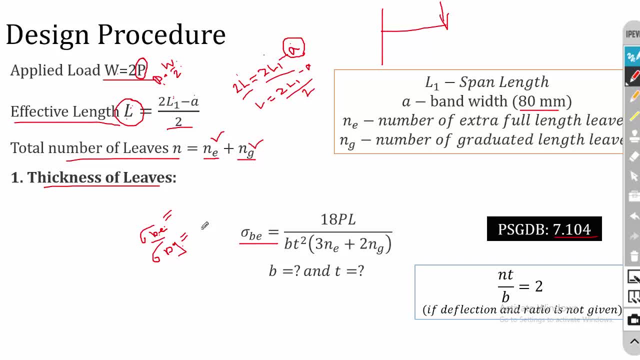 So that is why I have used B. E is for extra full length leaf and G is for graduated length leaf. So that is why I have used B. E is for extra full length leaf and G is for graduated length leaf. The extra full length leaves carrying 50 percent more load than the gradually length leaf. 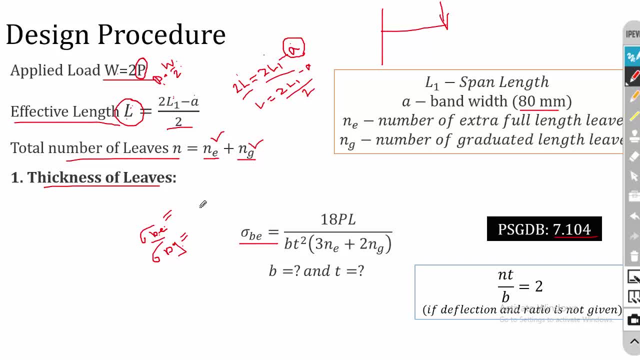 And while designing we have to focus on the maximum load condition. that is why we have selected the sigma BE. So this is subjected to heavy amount of load. that is why I have selected for designing. So sigma BE is equal to 18PL divided by BT square 3 NE plus 2NG. 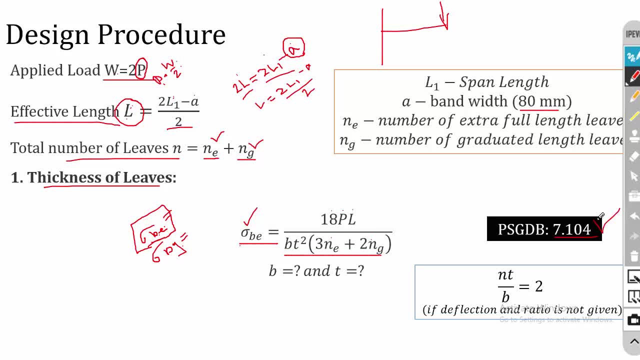 So this equation is there in the entire diagram. equation is there in data book, page number 7.104. so here p is the load applied, l is the effective length. so that we have calculated. that is why I have calculated the value of p and l in the earlier stage. then b is the breadth of the spring. so if this is the cross, 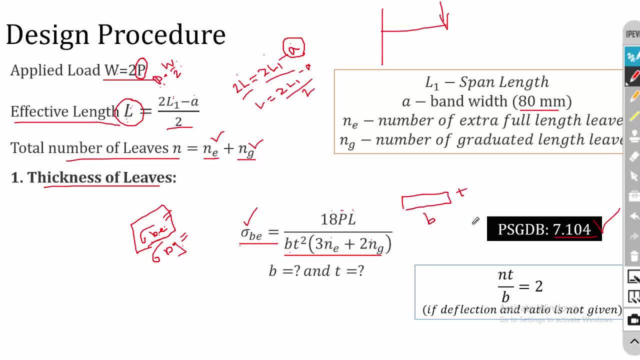 section. then b is the width and t is the thickness. so b and t we have to calculate. ne is extra full length leaf and g is graduated length leaf. so sigma b is material property. if it is given in the problem then we can take that or otherwise we can select a suitable material. 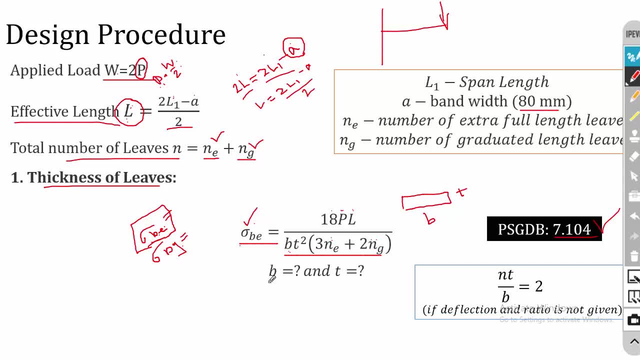 and we can assume some suitable stress values. so we have to calculate the b and t value. in most of the problems the ratio between the b and t value will be given. so if the ratio is not given, sometimes they may give the deflection value. so if the deflection 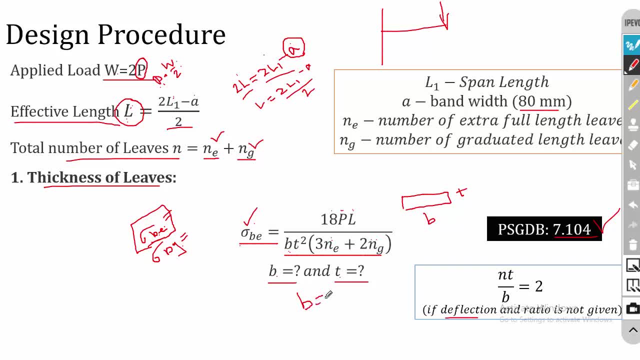 value is given. from this you can find the ratio, that is, b is equal to 1.5 times of t or 2 times of thickness. and by substituting the ratio in the upcoming equations we can calculate the b and t value. but if the deflection and the 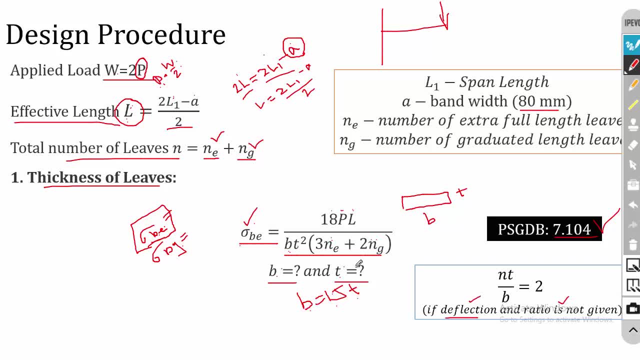 ratio, that is, ratio between width to depth, is not given, then we can assume a ratio of nt by b is equal to 2. so remember that if these two data are not given, that is deflection and ratio. So if these two data are not given in the problem, then we can assume a ratio of nt by 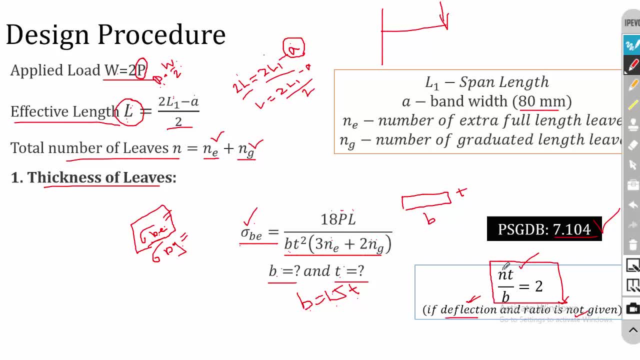 b is equal to 2. so here n is the total number of leaves, t is the thickness of the leaf and b is the width of the leaf. so by substituting this ratio in the equation we can calculate the value of b and t. so that is breadth and thickness. so after calculating the breadth, 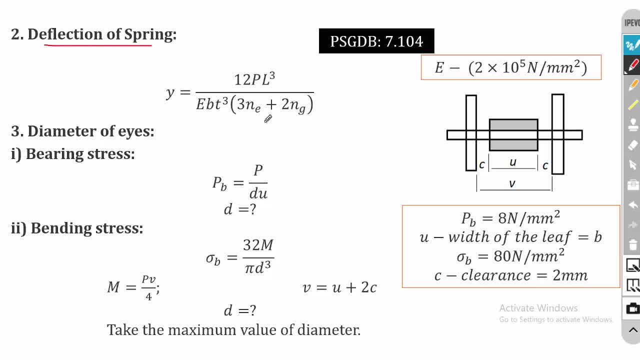 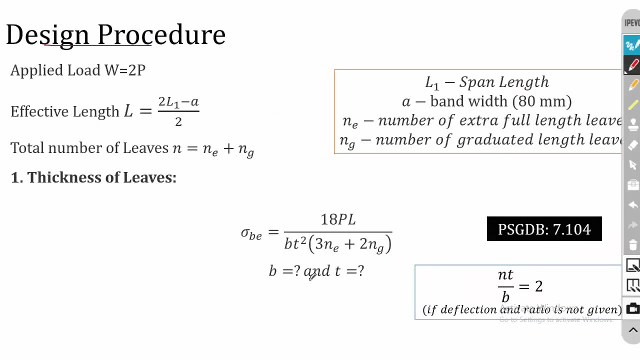 and thickness. then the second one is deflection. So, as I told earlier, In sum of the problems they will give the deflection value. So if the deflection value is given, then you do not need to assume the ratio because in the previous stage you will get b o okay. so if the deflection is given here you will get. 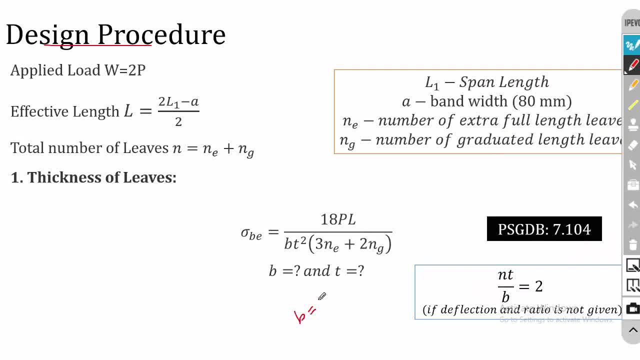 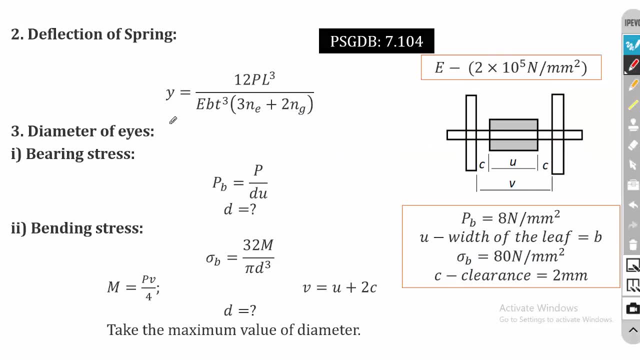 the ratio between b and t by solving this equation. That is its value. for example, we have considered b is equal to 1.5 times of the thickness. Now let us look at the problem. So if the deflection is given in the problem, then you can substitute: 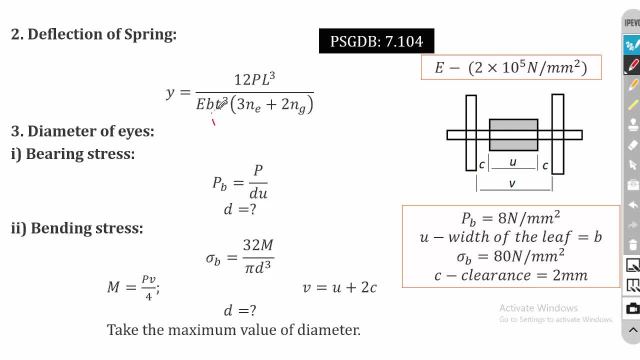 the value of b, that is, b is equal to 1.5 times of thickness. in this equation and substituting the remaining values, you can calculate the b and t. But if the ratio is given in the problem, or if we have assumed the ratio between b and t, then you can calculate the deflection value and you can write. 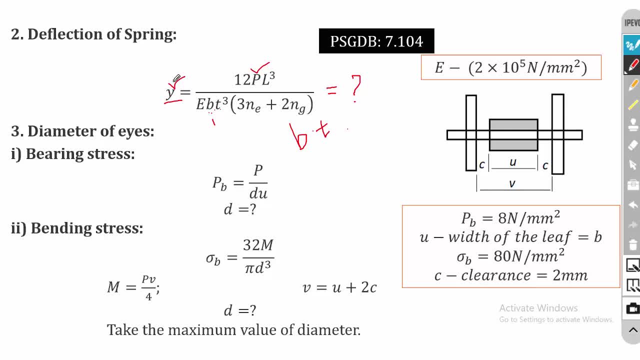 it here. So if the deflection is given in the problem, then by using the deflection you have to calculate the b and t. If the deflection is not given in the problem, then you have to calculate the deflection. So that is the second step. This equation is also available in the 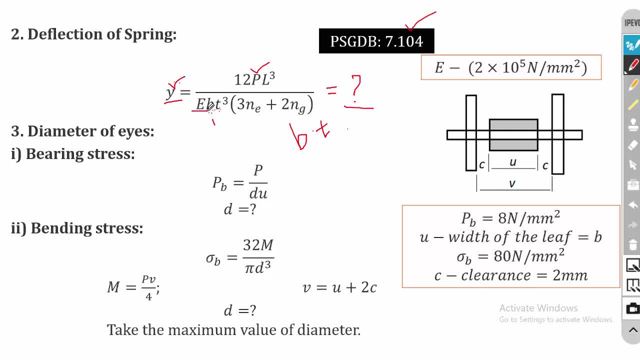 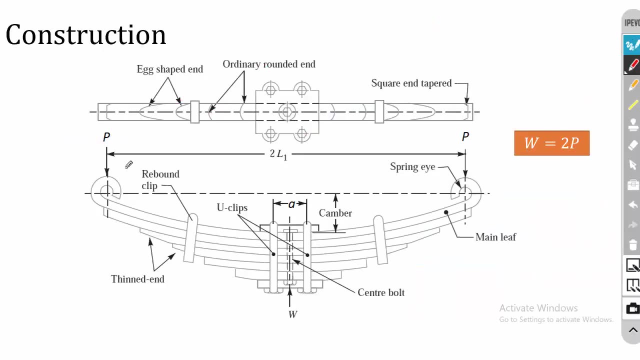 data book, page number 7.104.. So here e is the Young's modulus. So the Young's modulus of the spring material. The third step is diameter of the eyes. So in leaf spring you can see the eye here. So this is the eye bolt. So this eye bolt is used to clamp the leaf spring in the vehicle body. 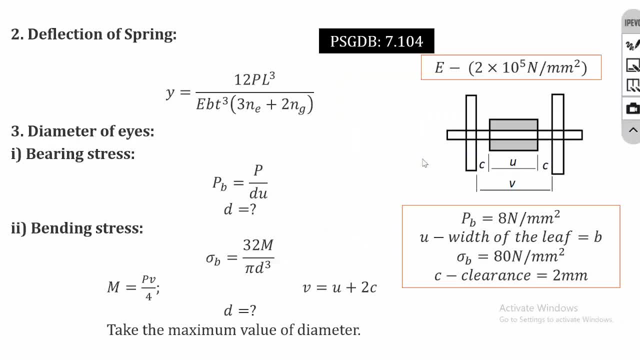 So this is the eye bolt. So this eye bolt is used to clamp the leaf spring in the vehicle body. So we have to design the eye bolt. that is the third step. So the eye bolt is subjected to two types of stress. one is bearing stress and another. 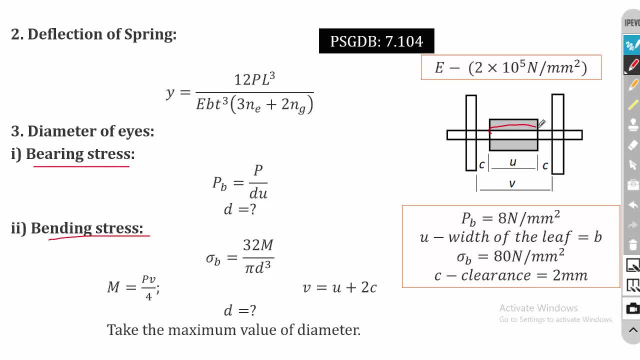 one is bending stress. So because of the compression between these two contact surfaces, bearing stress will be acting and because of the load acting on the leaf, a bending may occur in the eye bolt. So first let us consider the bearing stress. Pb is equal to P divided by D into U. that 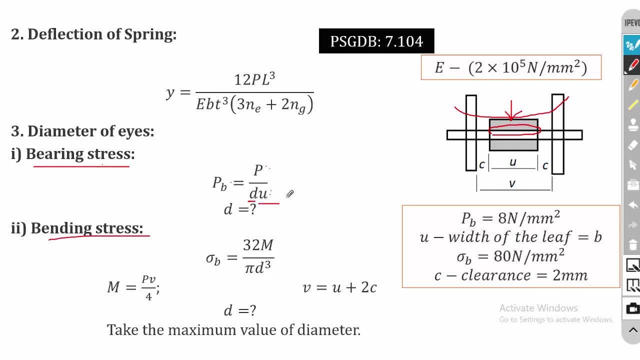 is the diameter of the bolt into the length of the bolt, U. So here you can see that U is the width of the leaf. width of the leaf: we have already calculated. that is equal to B, And if the Pb value is not given in the problem, we can assume a Pb value of 8N per mm2, you. 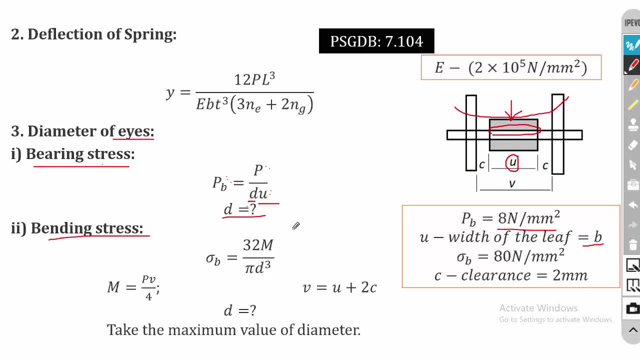 can substitute it and you can calculate the diameter of the eye. So this is the first possibility And the second one is the diameter of the eye is bending stress. we know that sigma b is equal to 32 m divided by pi d cube. and let 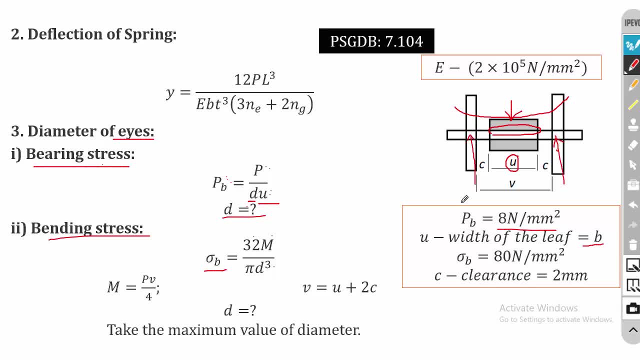 us consider this as a simply supported beam with the point load at the center. so m is equal to pv divided by 4. so here, if you see the drawing, you will get an idea about what is v. so v is the overall length of the bolt and v is equal to u plus c. that is clearance. 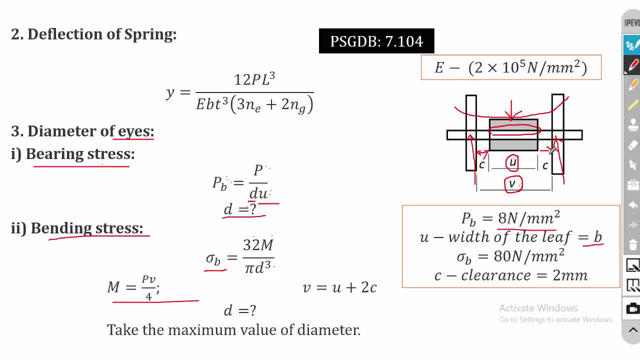 between the leaf and the support and in the right side you have another gap that is another clearance c. so the v is equal to u plus 2 times the clearance and the clearance value will be generally considered as 2 mm. so by substituting the clearance value and u value. 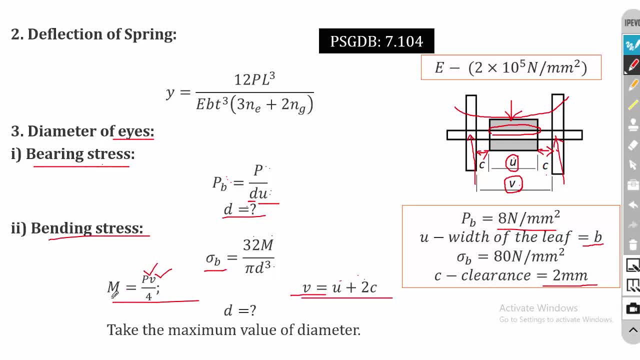 calculate v, then substitute the v value. p is the load acting. calculate the bending moment, then substitute the bending moment in this equation and calculate the value of d. so now you have 2 m, two diameter values. one is by considering the bearing stress and the another one is: 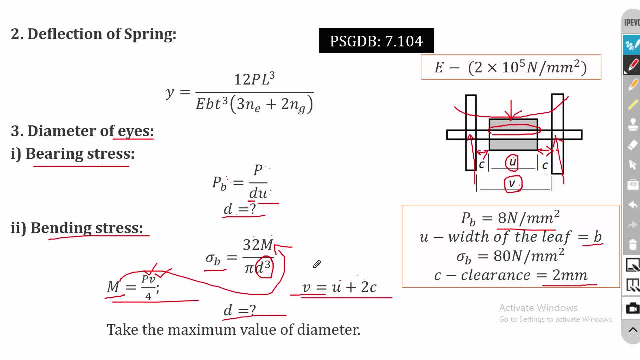 by considering the bending stress. so among these two you just take the maximum diameter. ok, so you can take the maximum diameter as the diameter of the eye bolt. so this is the third step. so third step will be somewhat confusing, so be clear about it. then the fourth. 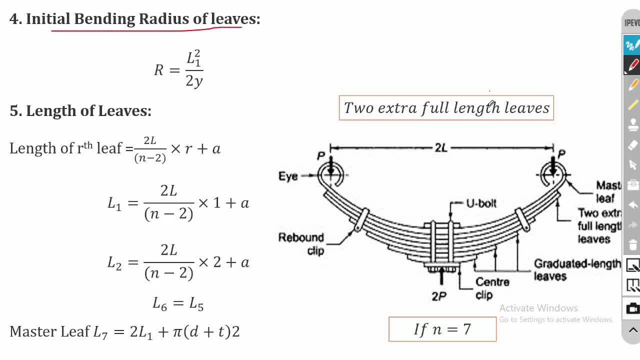 step is initial bending radius. so this is the initial bending radius. so that is, r is equal to l1 square divided by 2y. l1 is the overall length, span length, and y is the deflection. you can substitute it and you can calculate the value of r, the 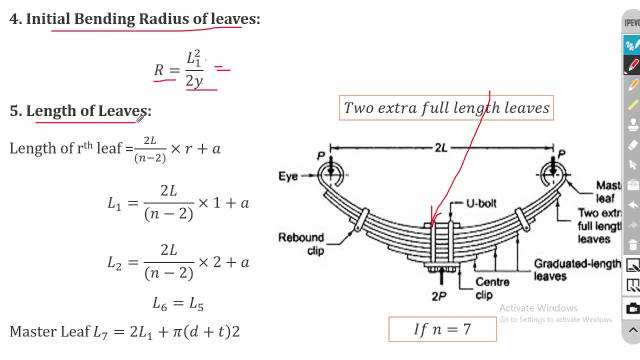 last step is length of the leaves. so if you have 7 leaves, then you have to calculate the length of all the 7 leaves. if you have 15 leaves, then you have to calculate the length of all the 15 leaves. so here for explanation, I have considered two explanations for the. 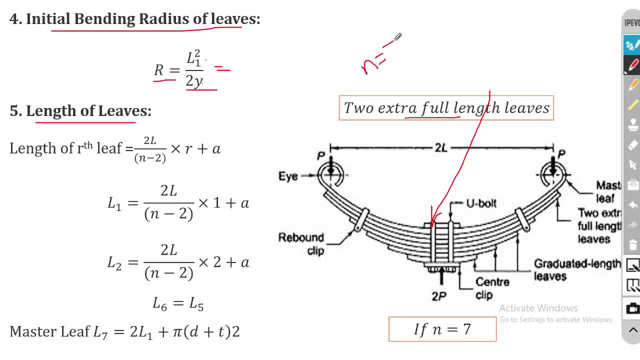 extra full length leaf, that is the overall length. overall number of leaf is n is 7 and ne is equal to 2. I have assumed so. actually, here I have assumed some data for explaining these procedures in a simple manner. so if ne is equal to and n is 7, then the gradual 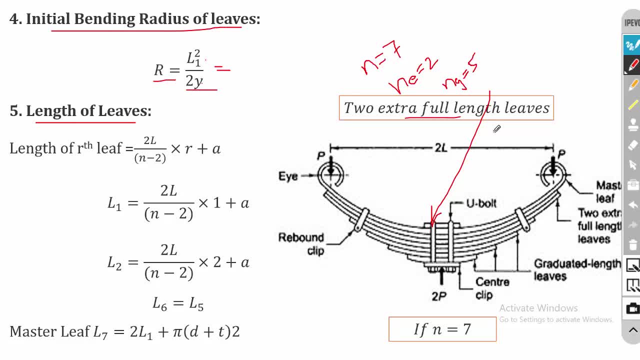 length leaf ng is 5, so 2 plus 5 is equal to 7. so the equation for calculating the length of the rth leaf is 2l by n minus 2.. this n-2 is, for ne is equal to 2.. So if ne is 3 then you have to use 3 here and r is 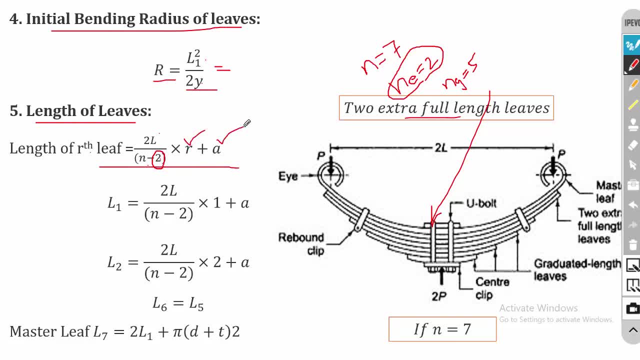 the number of leaf and a is the bandwidth. So here you can see that. so the bottom most one is it is l1, then l2, l3, l4 and we have two extra full length leaf, that is l5 and l6.. So l5 and l6 are two extra full length leaf, which means the length of l5 and l6 is 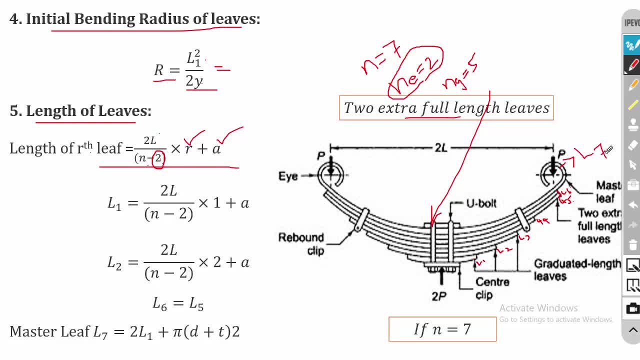 same and the last one is the master leaf, that is l7.. So if you have 15 springs with two extra full length leaf, then l15 is the master length leaf, l13 and l14 is the two extra full length leaf, that is, l13 will be equal to l14 and the remaining are graduated length leaf. 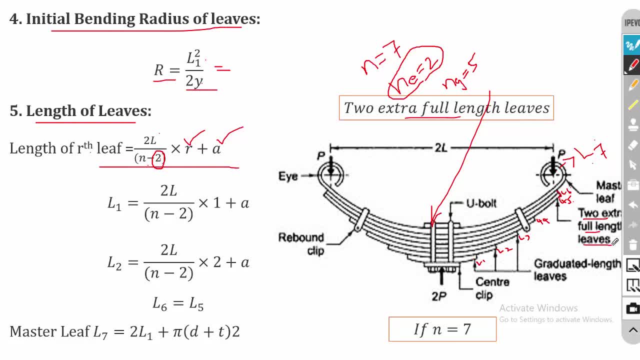 Here I have considered seven leaf with two extra full length leaf. So l5 and l6 are two extra full length leaf, So the l7 is master leaf. So the equation for calculating the master length is: l7 is equal to 2l1 plus pi into d, plus t into 2.. So d is the diameter. 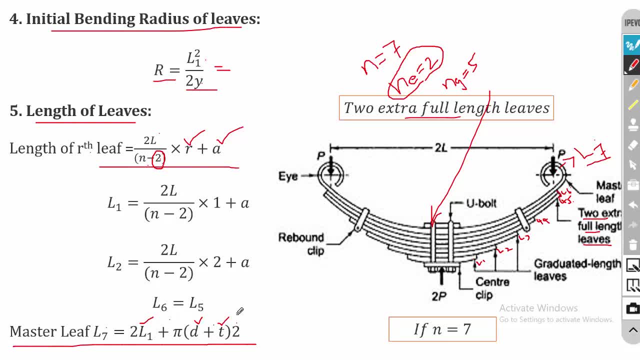 of the eye bolt. t is the thickness of the spring. I mean thickness of the leaf. So l7 is the master leaf. after that we have two extra full length leaf, that is l5 and l6, and we know that l6 is equal to l5 and l6 are two extra full length leaf, So l7 is equal.